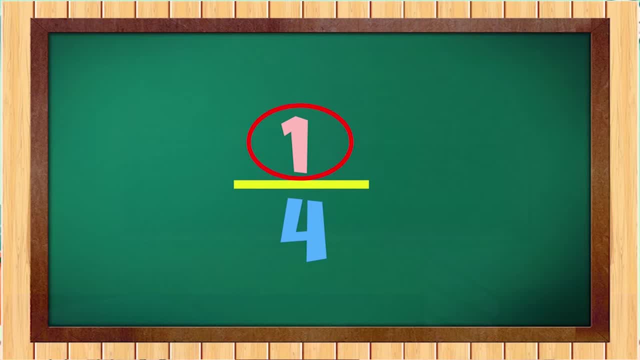 A fraction has two main parts: the numerator, which is the top number, and the denominator, which is the bottom number, And those two numbers are separated by a vinculum line. Now let's discuss the denominator. The denominator of a fraction tells us how many. 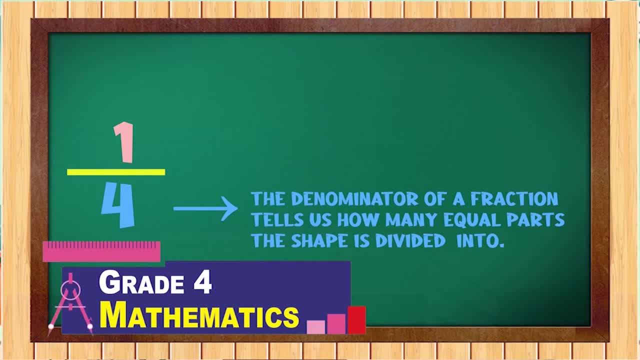 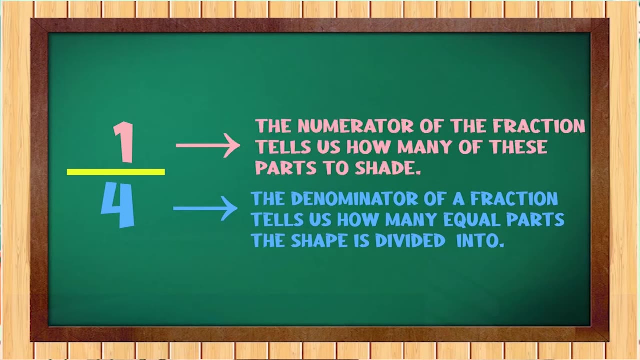 equal parts the shape is divided into. I repeat: the denominator of a fraction, which is the bottom number, tells us how many equal parts the shape is divided into, While the numerator, which is the top number, tells us how many of these parts to shade. This is extremely important when you're learning about shading and labeling. 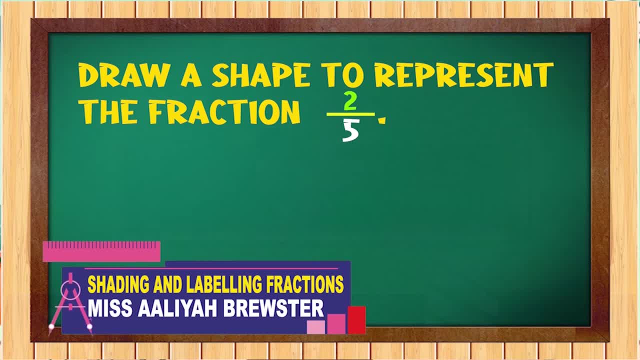 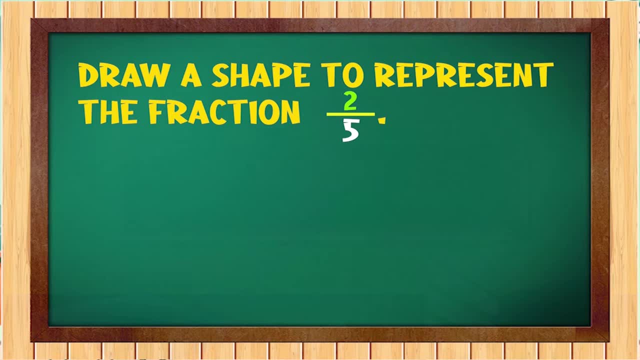 fractions. So keep that in mind. Let's work together. Take your notepad and draw a shape. Take your notepad and draw a shape to represent the fraction 2, fifths. Here's an illustration of any character's top number. He's very happy to have many musical values. 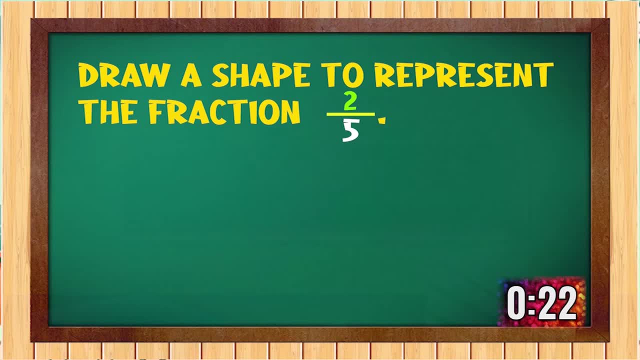 The rules are roped in well in reference to the proportion of udah après and after each score and number of favorites within the historic ratio. We don't say c-1 as something that's too far away, as something just comes to mind. 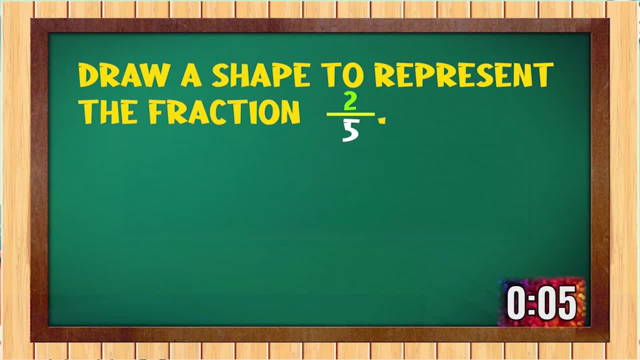 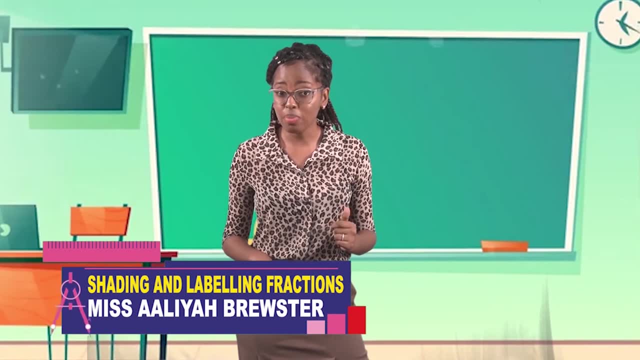 And we have to, و, for example, z-1.. So we're just going to plug in 4th And we're going to close ourologists two. Now that you're finished drawing your shape and divided it equally, let's discuss what this means. 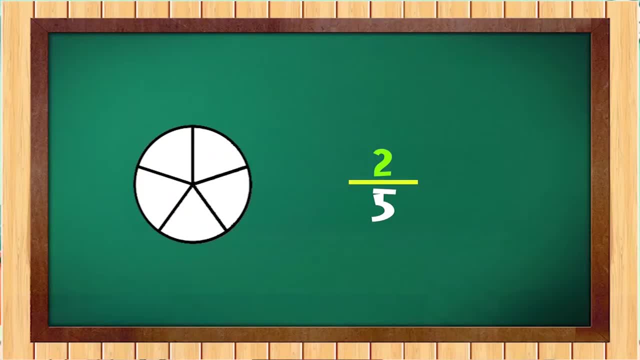 I'm going to use the shape of a circle. The denominator of 5 means that we have to divide our shape into 5 equal parts. So I would have divided my circle into 5 equal parts. The numerator of 2 means that we have to shade 2 parts out of the 5 parts. on the shape, I 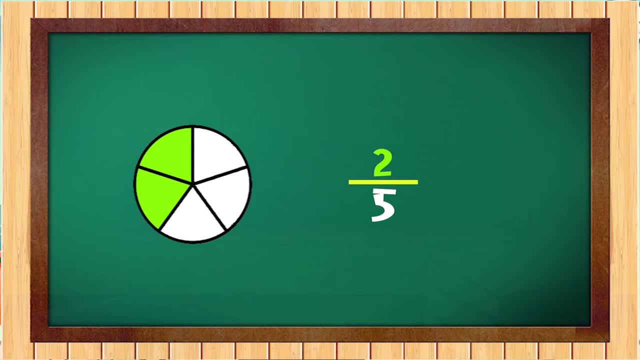 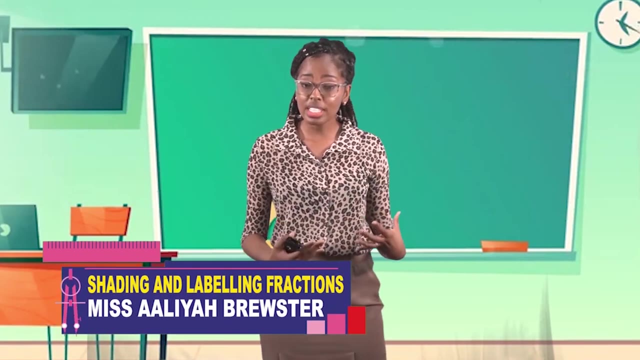 would have shaded 2 parts close together. However, it does not matter which 2 parts of the shape is shaded: it still represents the same thing. To continue, we're going to work some examples together. For these examples, we're going to look at how to shade and label. 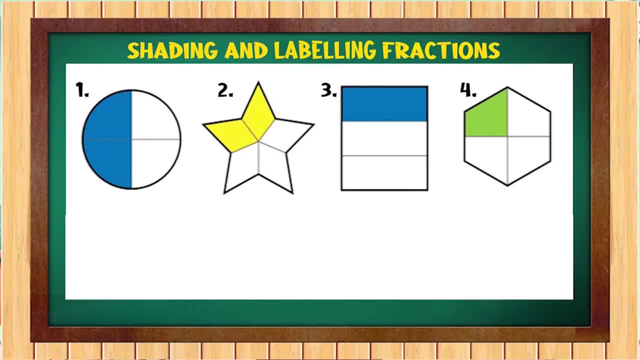 fractions. The first example is a circle. The circle is divided into 4 equal parts, and 2 out of the 4 equal parts are shaded. How do we label that shape as a fraction? Well, the numerator tells us how many parts are shaded, while the denominator would tell us how many parts. 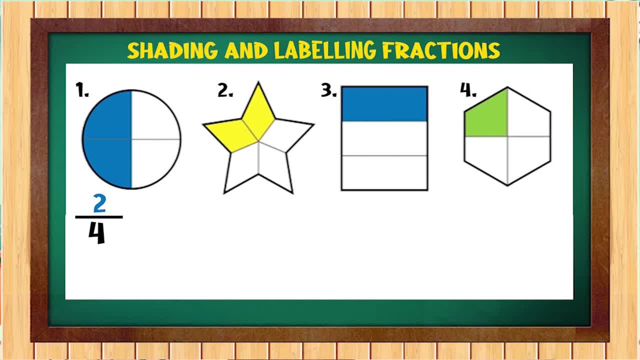 the shape is divided into. In this case, the amount of parts the shape is divided into is 4.. So 4 is our denominator, while the numerator, which is the amount of parts that are shaded, would be 2.. However, there's also another way to write that fraction. If you look at: 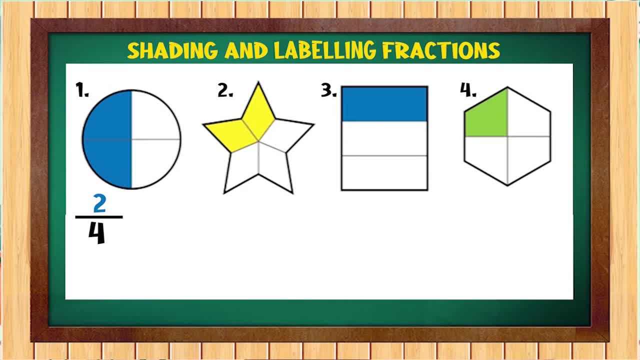 that shape properly. it's not just 2 out of 4 parts that are shaded. half of the shape is shaded. Therefore, 2 fourths can also be represented by a half. Now let's look at the second example. We have a star. 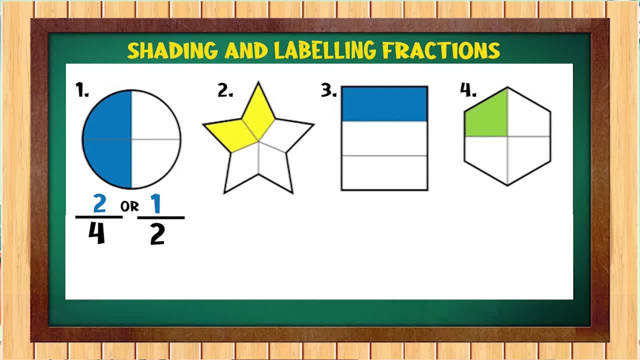 It's divided into 5 pieces and 2 of those pieces are shaded. How do we represent that in a fractional form? Well, the fraction would be 2 fifths. Moving on to the third example, we have a rectangle that is divided into 3 pieces and 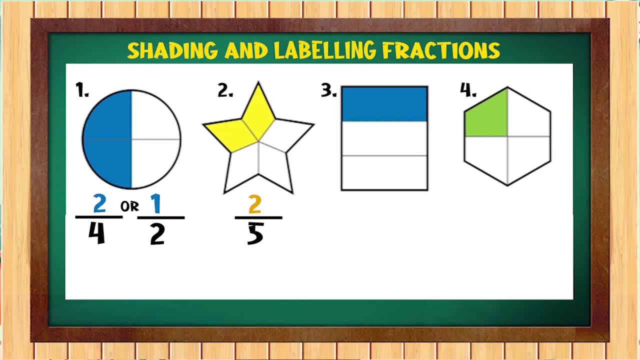 one of those pieces are shaded. We represent that shape by the fraction 1 third, because one part is shaded and the shape is divided by 1 third. The fraction is divided by one part and the shape is divided by one third. The fraction is divided by one third and 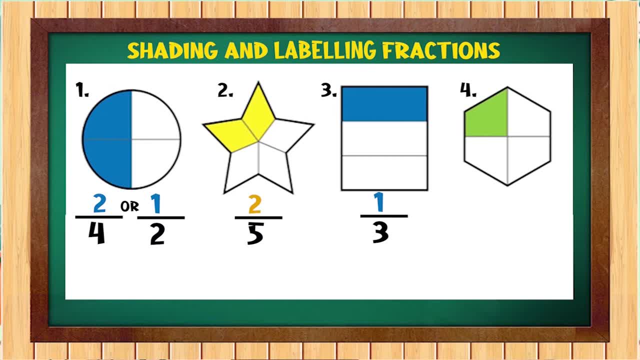 the shape is divided into three equal parts. Now let's do a fourth example. So this example is in the shape of a heptagon. The heptagon is divided into four equal parts, and one of those parts are shaded. If you guess the fractional part as a quarter, then you are correct. Now look at the. 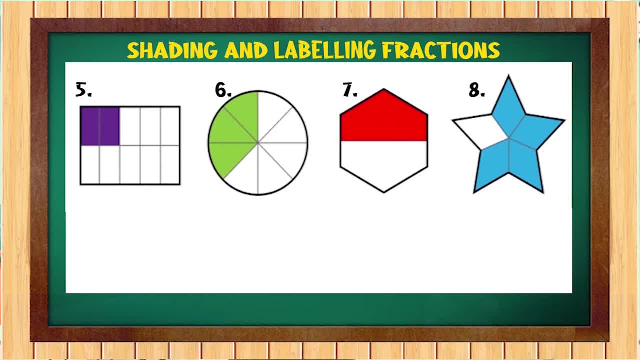 fifth example. Can you guess what the fraction for that shape would be? If you guess two tenths, then you are correct. That shape is divided into 10 equal piece and two pieces are shaded. Now let's look at our fifth shape. Look at it carefully and then identify a fraction. 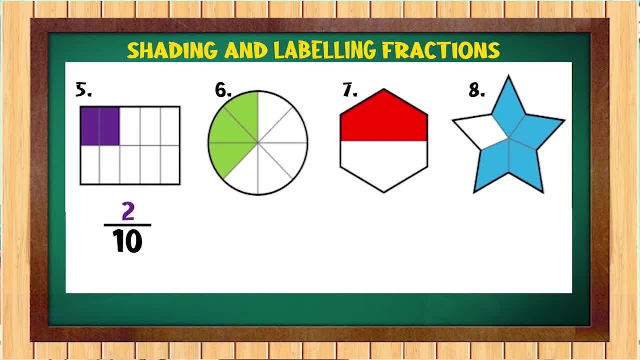 that would correctly represent that shape. Here the shape is divided into eight equal parts. It's a circle and it's cut into eight equal parts, and three out of those parts are shaded. The fraction, therefore, would be a quarter. If you guess the fraction for that shape as a quarter, then you are: 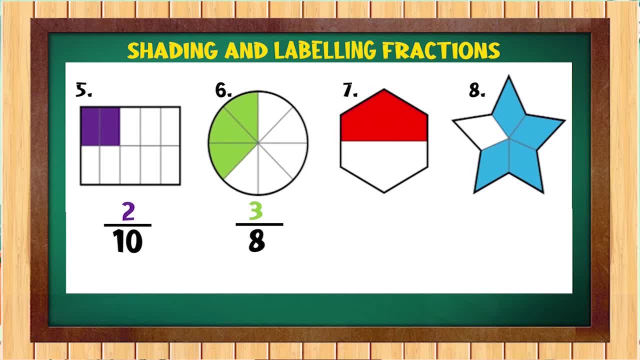 correct. The fraction, therefore, would be three eighths. So if you guessed three eighths, well done. Now let's look at our sixth example. This is also a heptagon and it's divided into two parts, and one of those parts are shaded. How would you represent that shape? Simple miss, one above two a half. 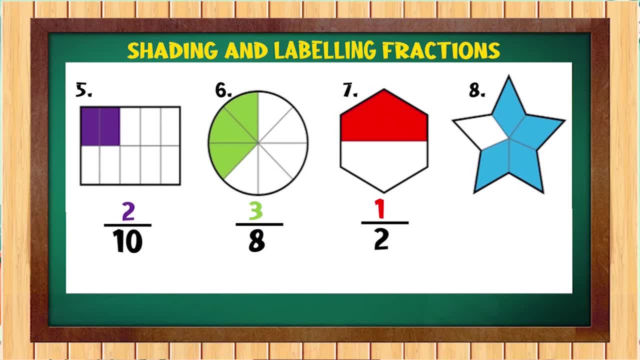 Well, if you guessed that, then you're definitely correct. To represent that shape, we use the fraction half. Now for our final example, we're using back the star, and the star is divided into five equal parts, and four out of those five parts are shaded. What fraction would you use to describe that shape? 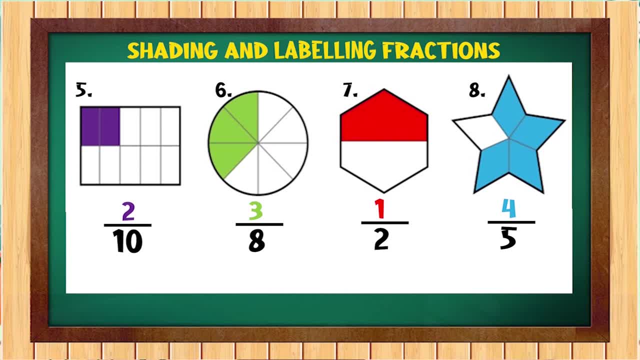 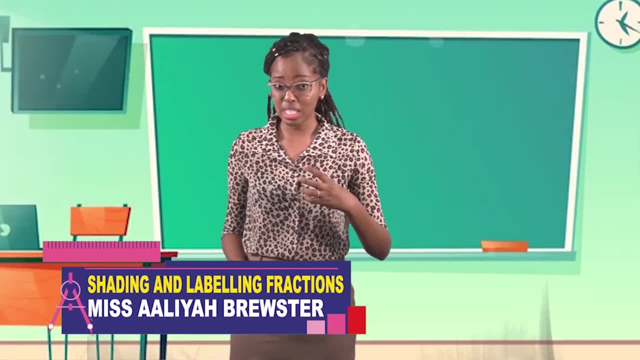 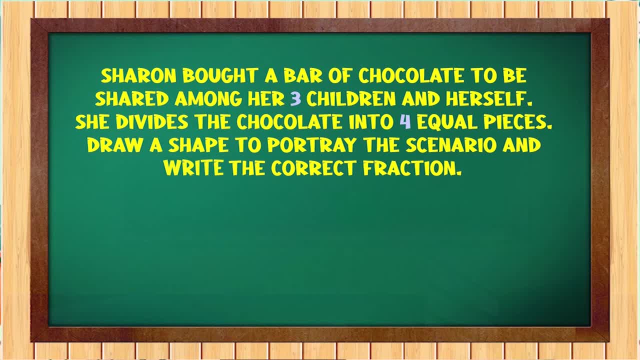 She bought a bar of chocolate to be shared amongst her three children and herself. She divides the chocolate into four equal pieces. She gives each child a piece of chocolate and saved one in the refrigerator for herself. Draw a shape to portray the scenario and write the correct fraction. 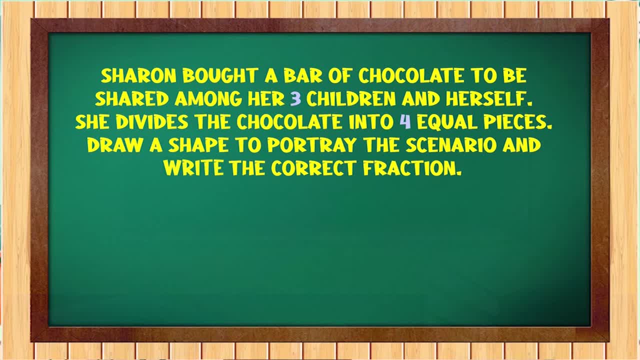 So this scenario is quite simple. To represent the bar of chocolate, we drew a rectangle. We divided the rectangle into four equal parts. Why? Because the scenario said that she bought the chocolate to be shared amongst herself and her three children. So that's four persons, right? So we divided our. 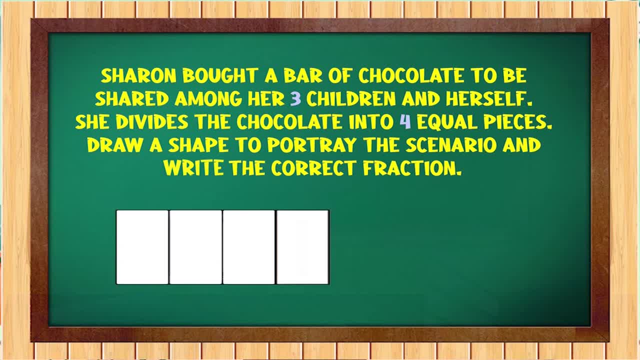 rectangle into four equal parts and it said: from the scenario we can infer that three parts were given to the children. So we shared three parts. So the fraction that would represent that shape would be three fourths, because the shape is divided into four equal parts. So we divided the rectangle. 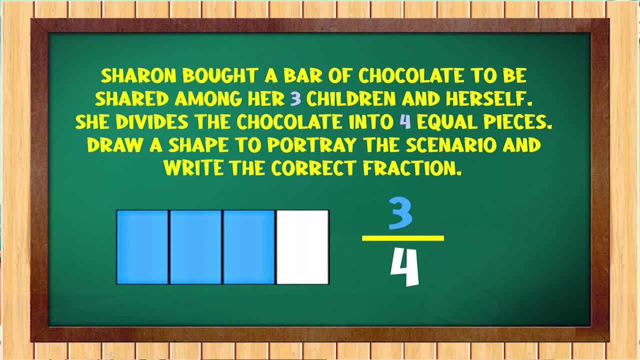 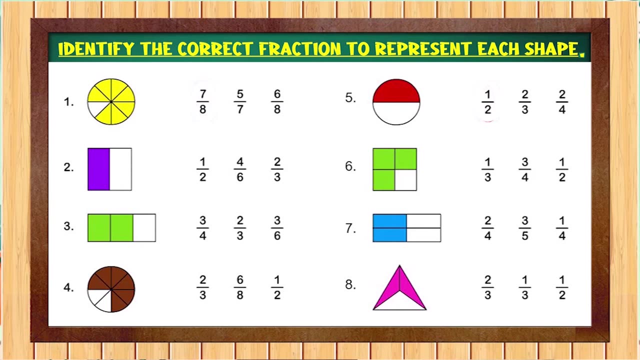 into four equal parts, The denominator would be four. The amount of parts that were shaded is three, So the numerator is three. It's time for you to do some activities on your own, But I won't leave you just like that. I'll do two for you and you'll do the rest For this activity you're asked to. 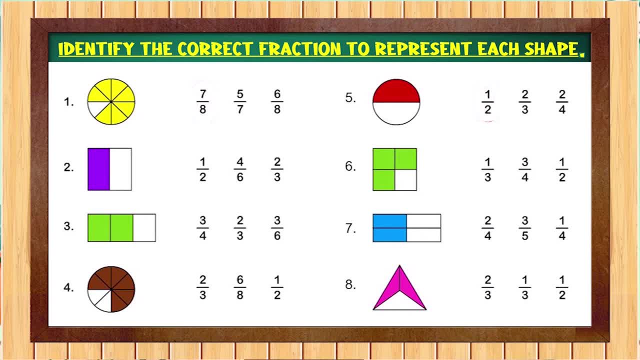 identify the correct fraction to represent each shape. So I'm going to do number one and number five. Number one: the shape is a circle. That circle is divided into eight equal parts and seven of those eight equal parts are shaded. From that I know that the fraction has to be seven. 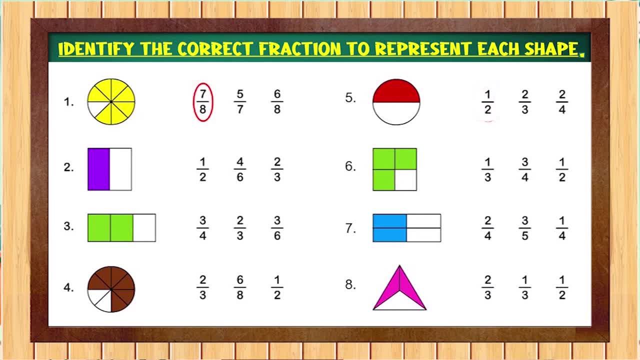 eighths, because seven is the amount of parts that are shaded and eight is the total number of parts that the shape is divided into. Good, Number five. now we have a circle, and the circle is divided into two equal parts. So we divided the rectangle into four equal parts. So we divided the rectangle. 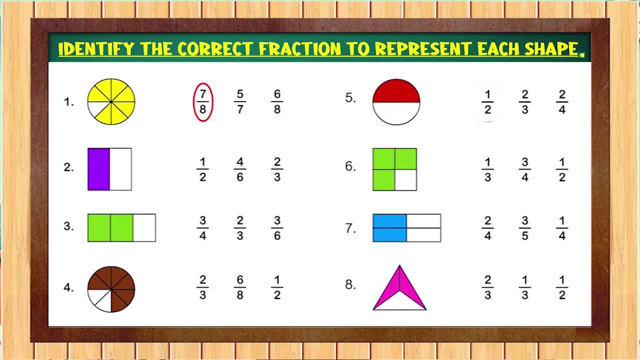 into four equal parts and one part is shaded. Now from that I know the fraction has to be half. Why? Because the denominator is two, because two equal parts The shape is divided into and the numerator is one because one of those parts are shaded. So that's the correct answer. So you, 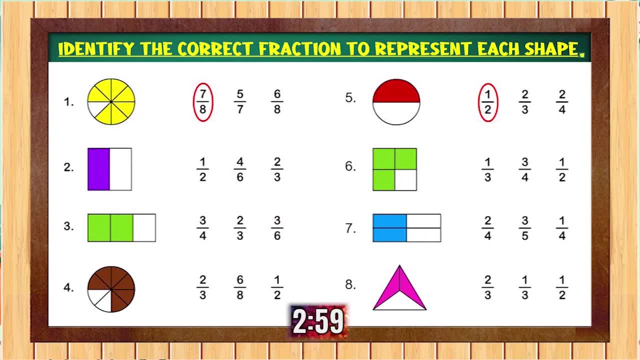 work the rest and I'll be back to discuss. Thank you so much for watching. I hope you enjoyed this video. I'll see you in the next one. Bye, Bye, Thank you, Thank you, Thank you. Are you able to get all correct? 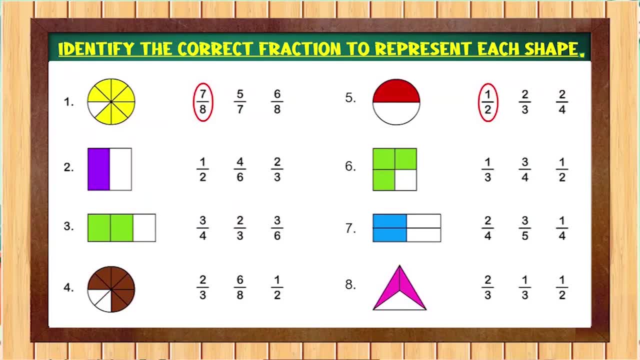 Let's verify. So for number two, we have a rectangle. there. The rectangle is divided into two equal parts, and one of those parts are shaded. Therefore, the fraction to represent that shape would be a half. Number three: there is a rectangle again, but this rectangle is divided into three equal parts, and two of those parts are shaded. 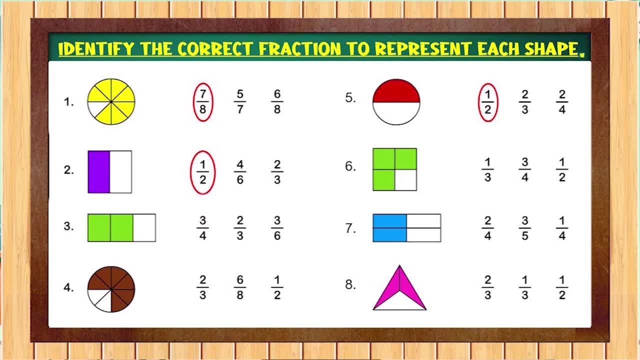 Therefore, the correct fraction to represent that shape would be two thirds. Number four: we have a circle. That circle is divided into eight equal parts, and six out of those eight parts are shaded. So the fraction to represent that shape would be six eighths. 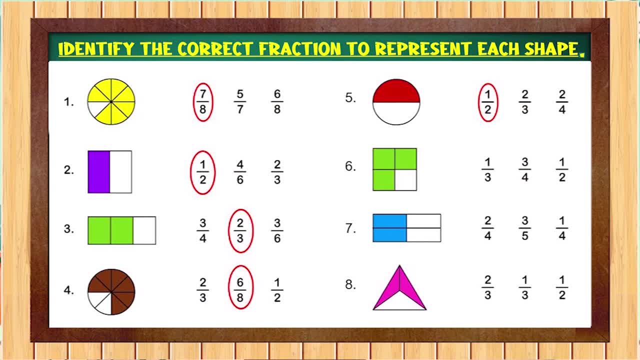 Number six: we have a square. The square is divided into four equal parts, and three out of those four equal parts are shaded. Therefore, the fraction to represent that shape would be three fourths. Number seven: There's a rectangle. The rectangle is also divided into four equal parts, and two out of those four parts are shaded. 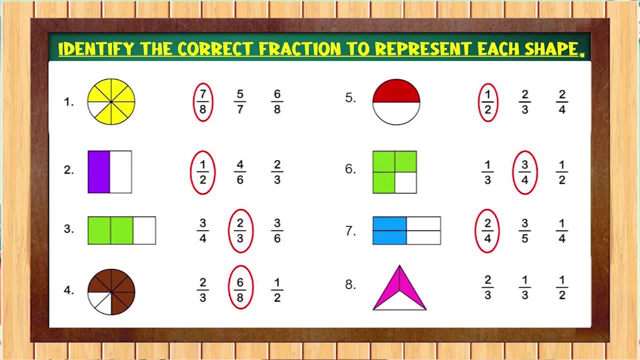 Therefore, the fraction to represent that shape would be two fourths or a half. The last one. we have a triangle, and the triangle is divided into three equal parts and two out of those three parts are shaded. The fraction to represent that shape would be two thirds. 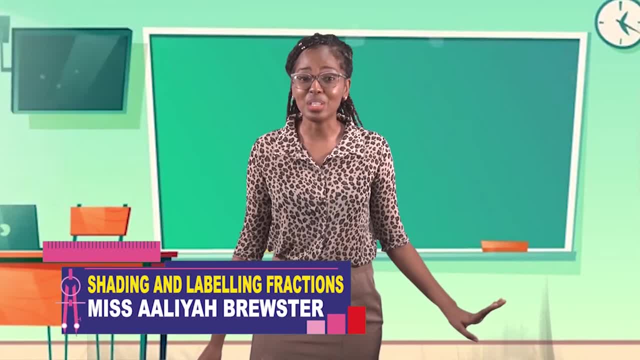 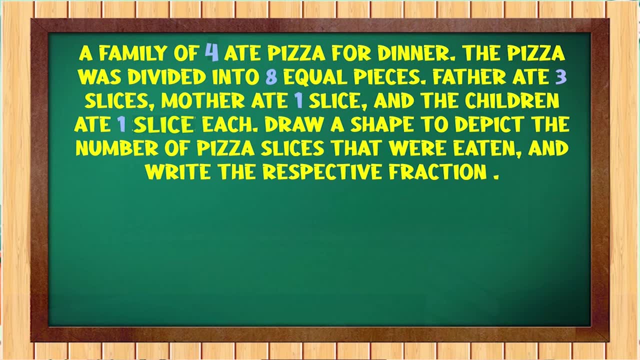 It's time for us to do one last activity. This is problem solving. The scenario says A family of four ate pizza for dinner. The pizza was divided into eight equal pieces. Father ate three slices, Mother ate one slice because she's watching her figure. 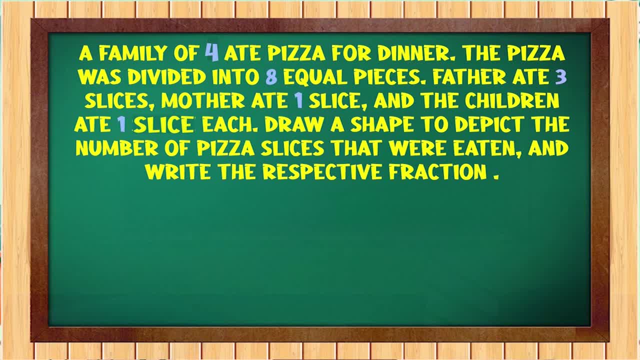 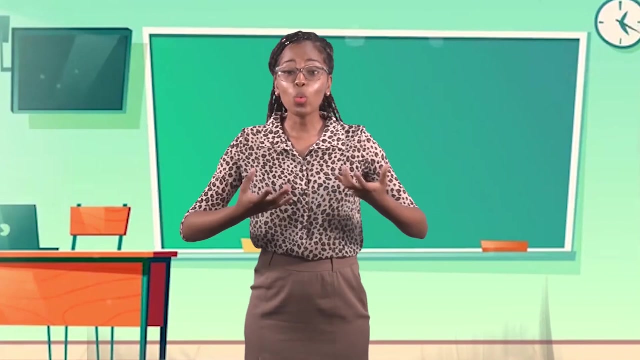